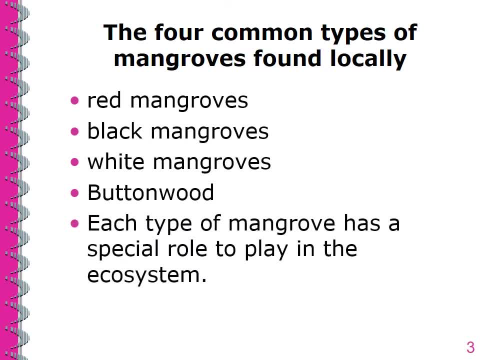 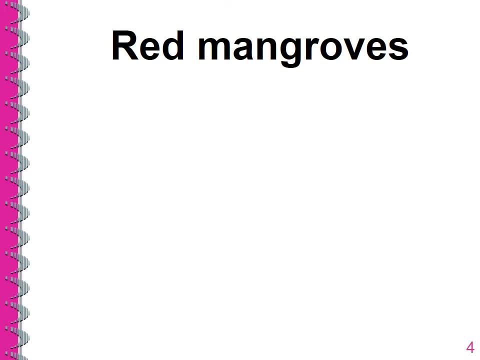 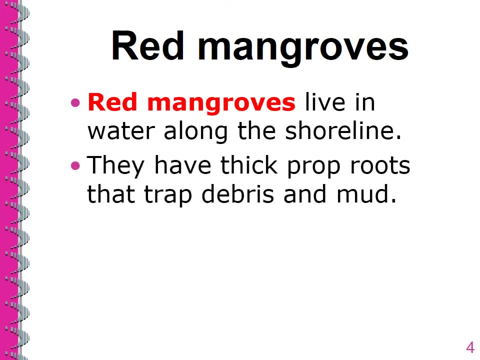 Each type of mangrove has a special role to play in the ecosystem. Red mangroves: Red mangroves live in water along the shoreline. They have thick prop roots that trap debris and mud. They help to prevent water from flowing inland and this helps to reduce flooding. 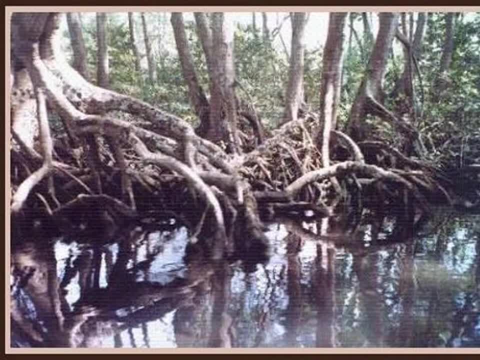 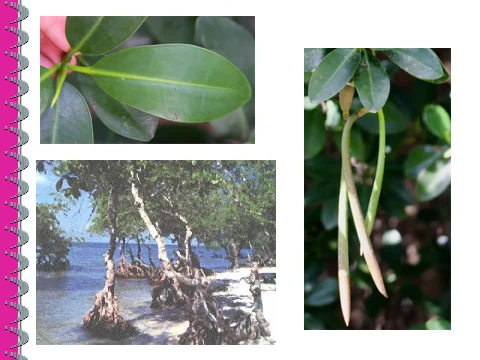 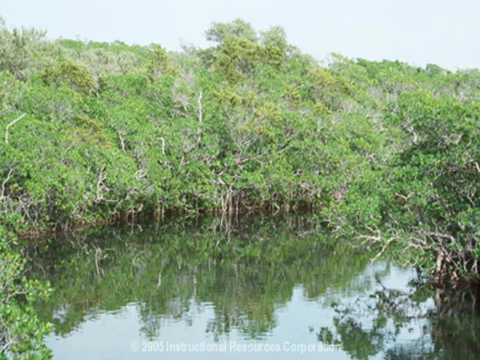 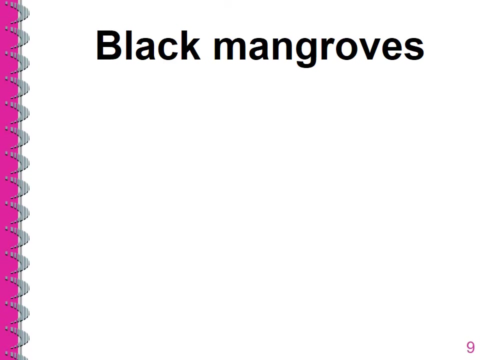 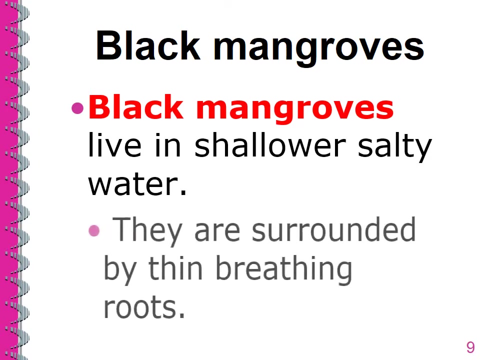 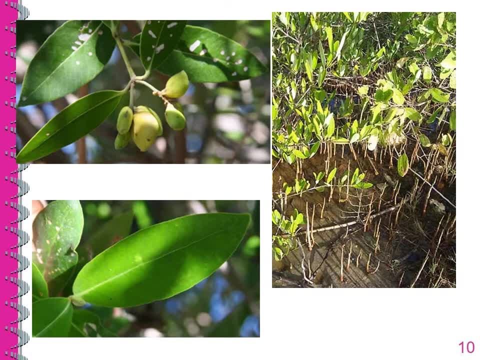 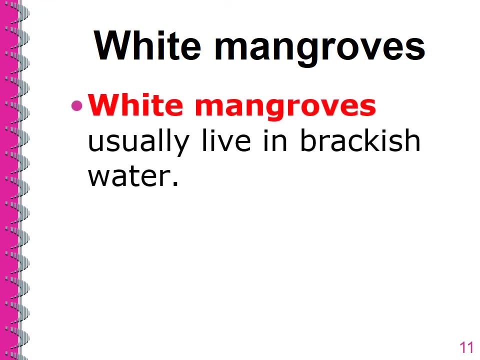 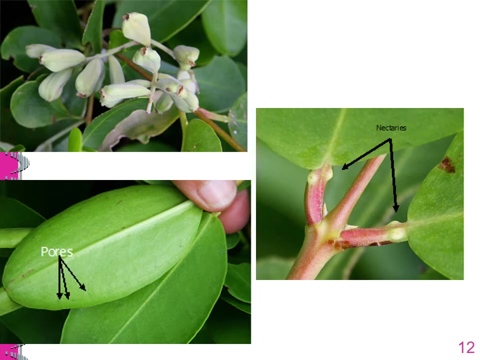 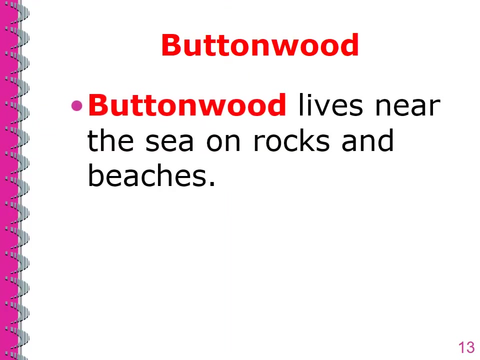 by thin breathing roots. black mangroves- the fruit, the flower, shallow water, white mangroves. white mangroves usually live in brackish water. they have thick, knobby breathing roots. white mangroves, buttonwood, buttonwood- live near the sea or on the beach. 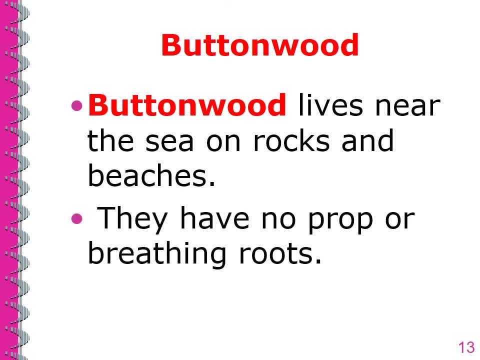 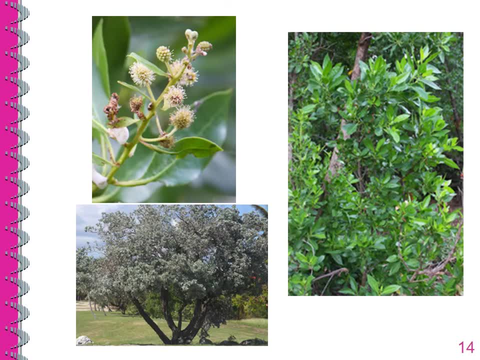 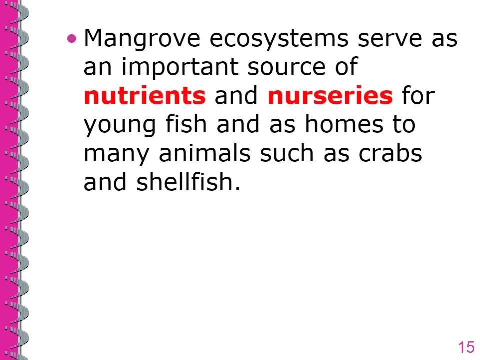 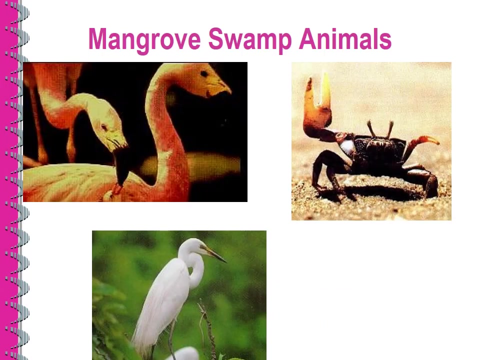 on rocks and beaches. they have no prop or breathing roots. buttonwood mangrove ecosystem serves as an important source of nutrients and nurseries for young fish and as homes to many animals such as the crab and the shell fish. in the bahamas, mangroves are referred to as flat swamps and slough squashed. 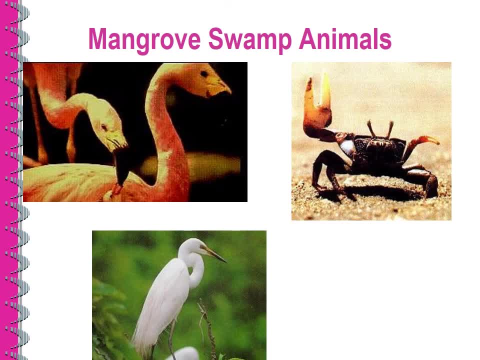 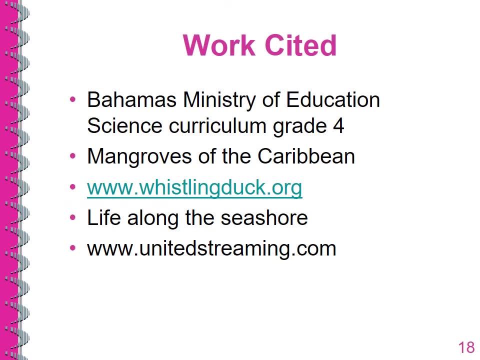 mango swamp animals: the flamingo, the egret, the crab mangrove, Spain. mangrove Beigno西 Rider Goldfish mangrove, South Waller Camel. History of species- unusual mangroves僕. Thank you. 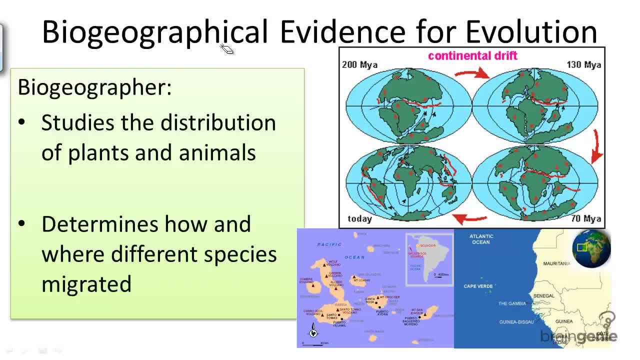 Biogeographical evidence for evolution. Well, to understand evidence for evolution in terms of biogeography, we need to understand what a biogeographer does. This is someone who studies the distribution of plants and animals on Earth. Just look at the breakdown of the word. 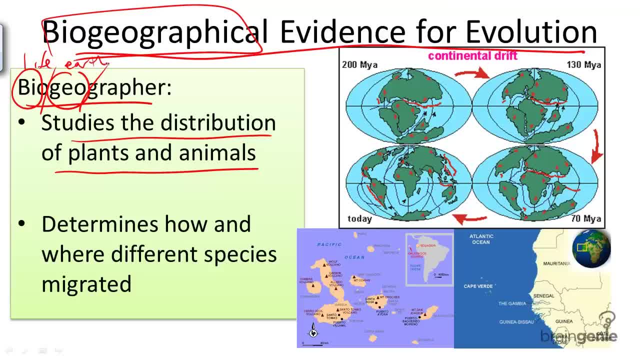 Bio means life, geo means Earth and graph means to write- Someone who studies or writes about life on Earth. So why is this important? Well, biogeography helps us to understand or explain evolution in terms of the fact that similar environments 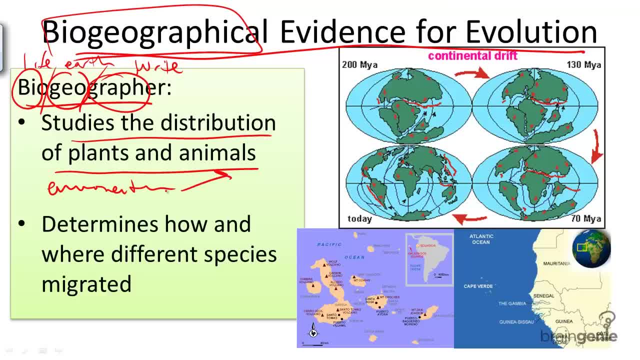 can lead to the evolution of similar organisms or animal species, even if the environments are really far away. So I'll put similar species that are far away. One example that can help us understand biogeography and be illustrated using Darwin's observations: 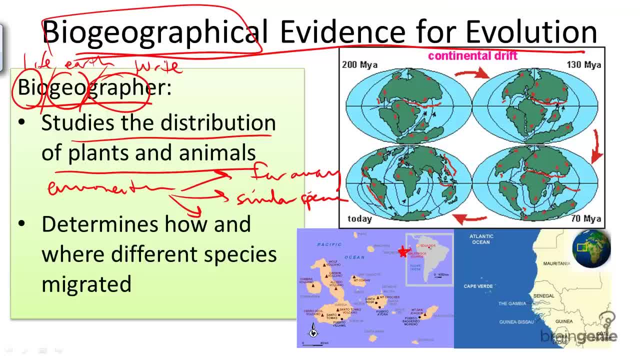 are the islands of the Galapagos, off the coast of South America, and the islands of Cape Verde off the coast of Africa. What he realized is that island organisms, even though they were both on islands, were actually more similar to their counterparts on the mainland than they were to each other.